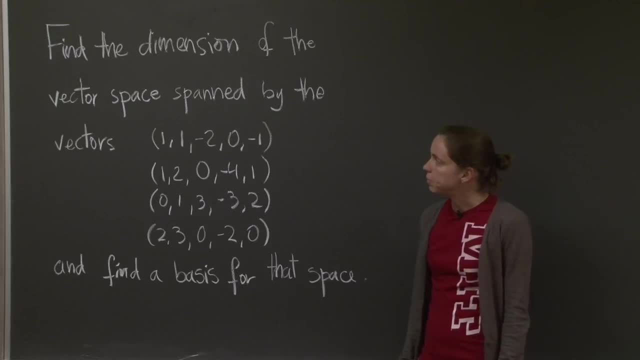 We're back, Let's work on it. Well, so we need to find the dimension and the basis. Remember what the dimension is. It's simply the number of vectors in a basis for the vector space. So actually the problem is backwards. We want to find the basis for the space first and then find the dimension. 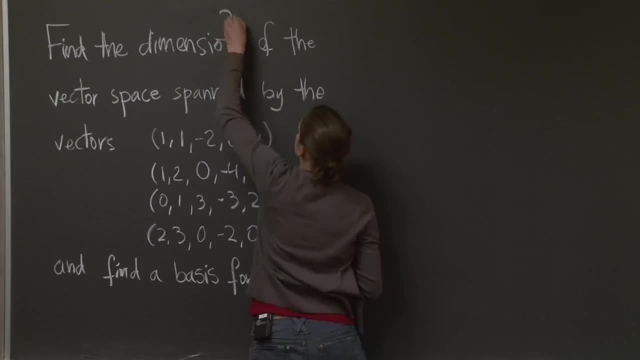 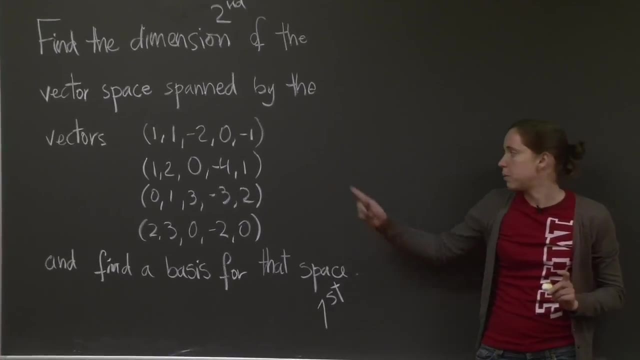 All right, All right, First here and second here. All right, So we want to find a basis for the vector space spanned by these four vectors. All right, All right. So we want to find a basis for the vector space spanned by these. 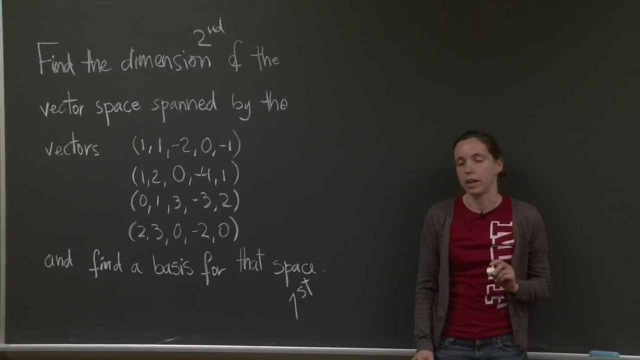 four vectors, All right. So you might be tempted to just say that a basis for this vector space is those four vectors, because they span the vector space. But there's another thing that a basis has to satisfy, and it is: the elements of the basis have to be linearly. 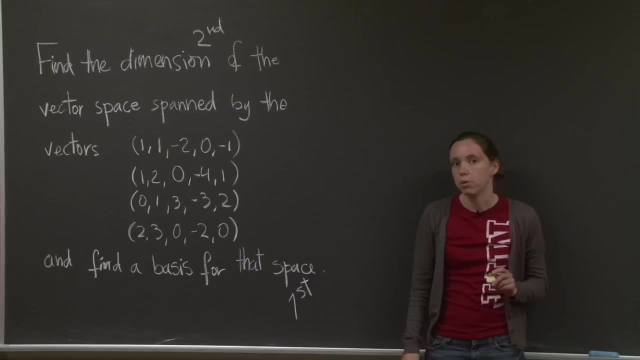 independent, And we don't know that these are. So we have to check. How do we check that four vectors are linearly independent? Well, there's a couple of different ways, But here's what we're going to do. We're going to put these vectors as row vectors. 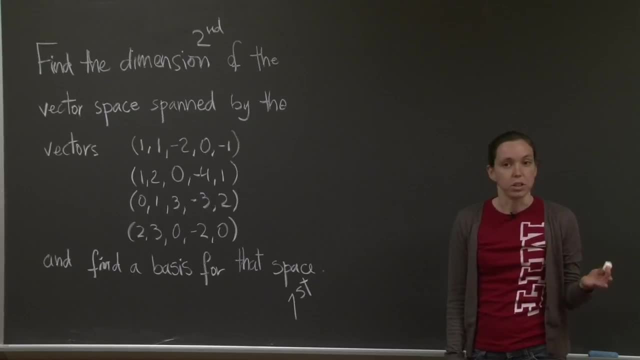 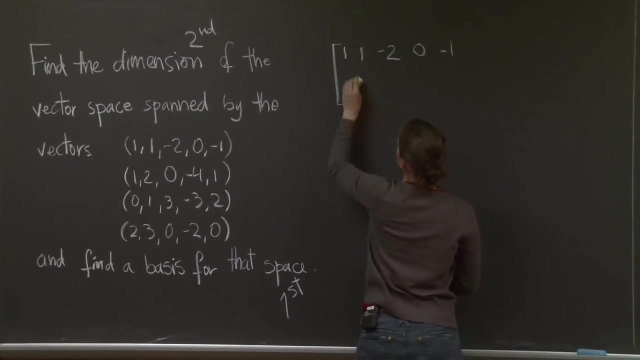 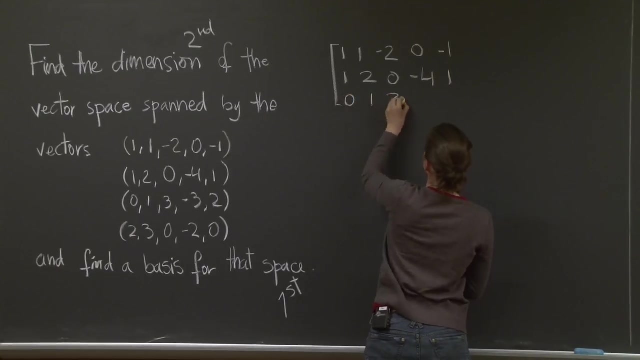 We're going to do rows of a matrix And then we'll do elimination, And when we get to the end, the rows that have pivots are the independent ones. So let's do that: 1, 1 minus 2, 0, minus 1, 1, 2, 0, minus 4, 1, 0, 1, 3, minus 3, 2, 1, 2, 0, minus 4, 1, 0, 1,. 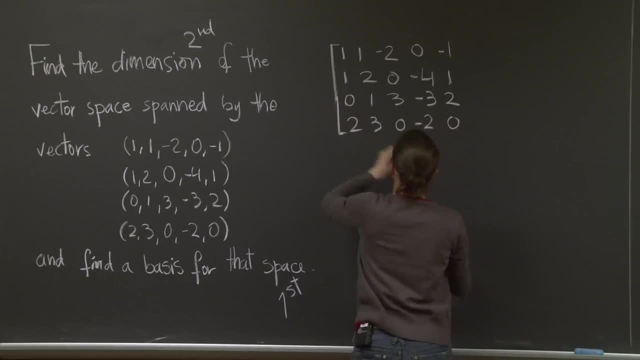 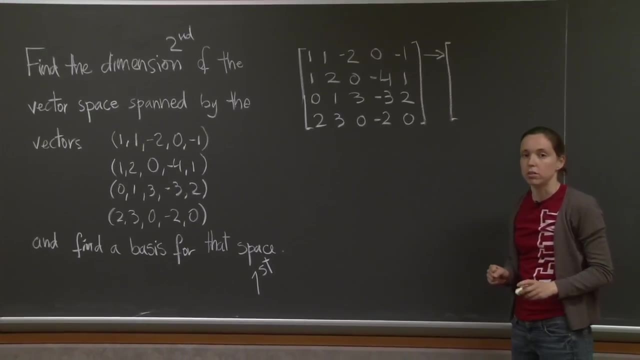 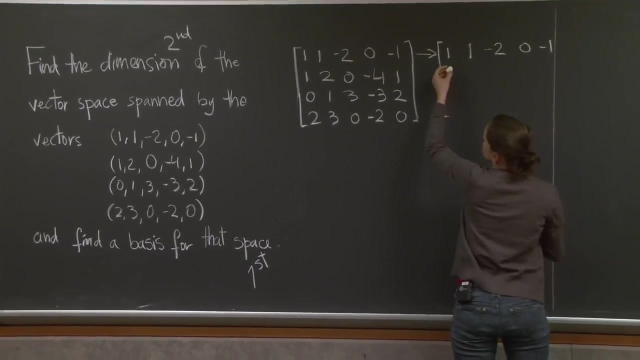 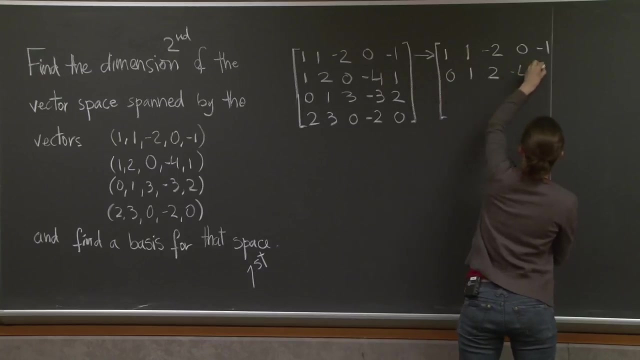 3, 0, minus 2, 0.. All right, By now you must have done elimination a million times, So I'll go a little bit faster: 1, 1 minus 2, minus 1, 0, 1, 0, plus 2, minus 4, 2.. This: 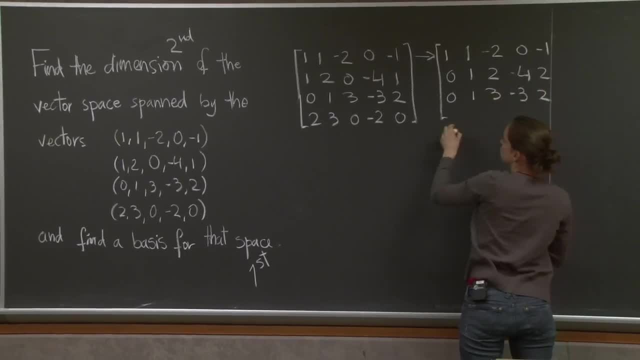 one's already done: 1,, 3, minus 3,, 2.. 2, minus 2,, 2, minus 2,, 3, minus 2,, 0, plus 4, minus 2, and 2.. 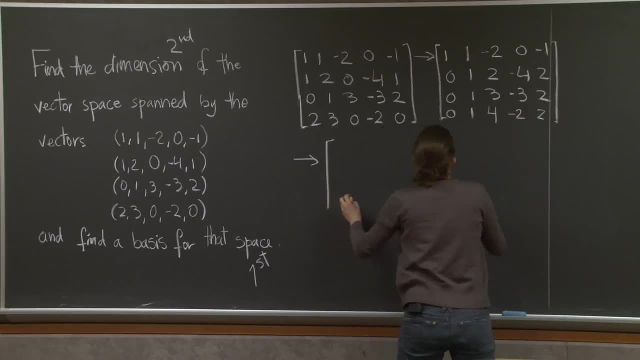 All right, One more step: 1, 1, minus 2, 0, minus 1, all these are done: 0, 1, 2, minus 4, 2, 0,. oh, 1 minus 1 is 0.. 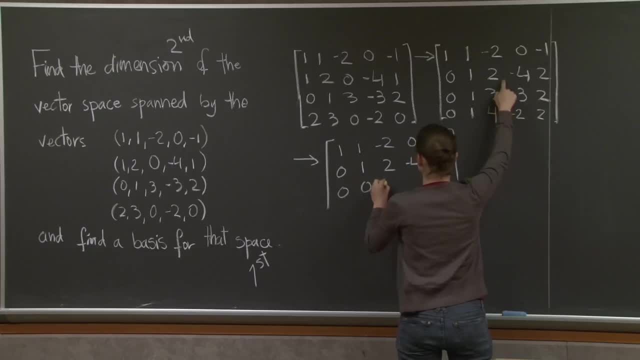 All right, Can I do it again? Yes, row 3 minus 2 is 1.. Minus 3 plus 4 is 1.. 2 minus 2 is 0.. 1 minus 1 is 0.. 2, 2 again. 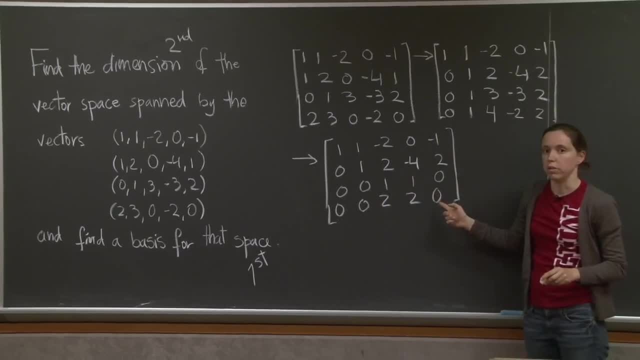 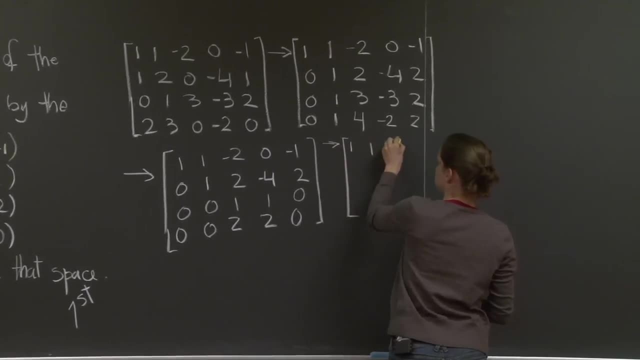 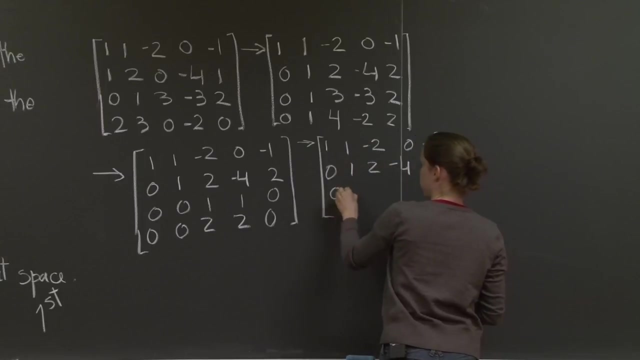 and 0.. Oh, you can see where this is going. In the next step, this row is going to disappear: 1, 1, minus 2, 0, minus 1, 0, 1, 2, 2, 0, 0, 1, 1, 0, 0, 0, 0, 0, 0, 0.. All. 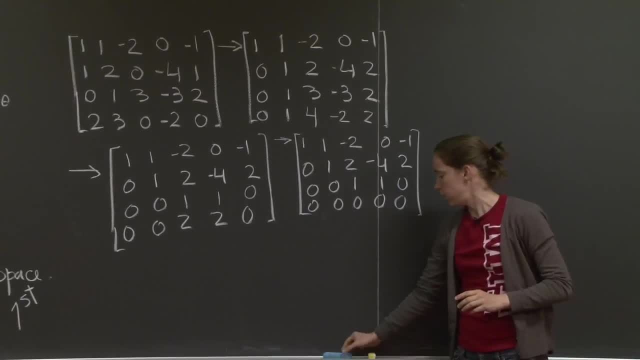 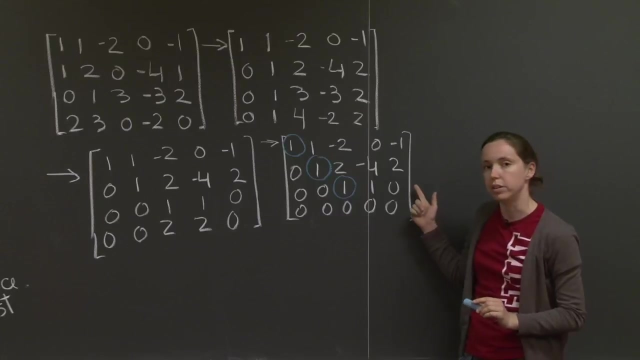 right, We're done with elimination, And so let's circle our pivots. Here are our pivots: We have three pivots, And so these three rows are linearly independent And in fact, these rows still span the same space that the initial four rows did. Because when you do elimination, 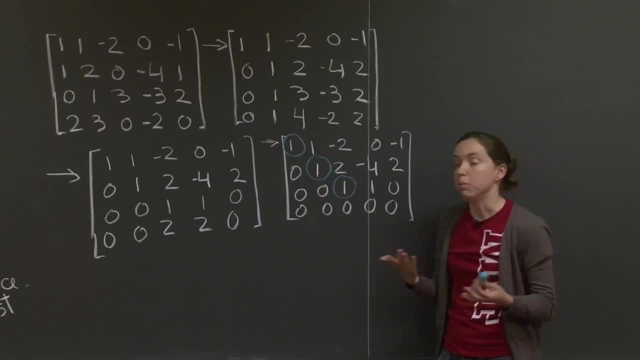 all that you're doing is recombining your rows by doing linear combinations of them. So, for example, your first row stayed the same throughout. Your second row was replaced by row 2 minus row 1.. But it's really still spanning the same space. And it goes on. And then the fourth row it. 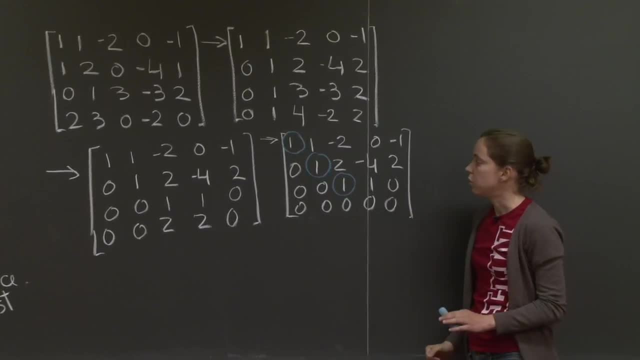 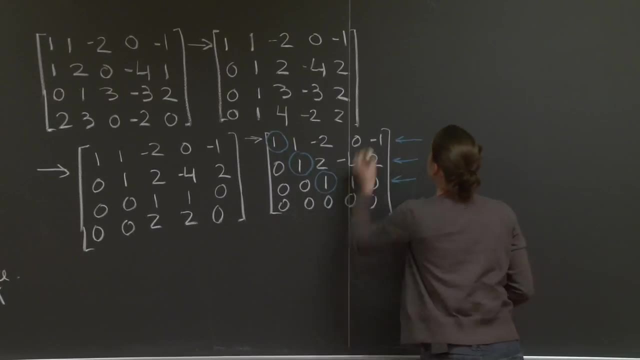 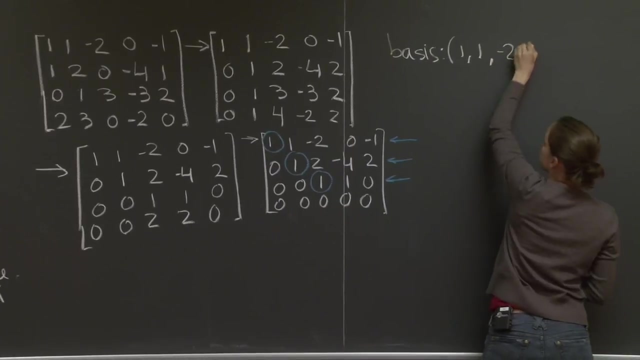 turns out was useless. You only needed the first three. So the elements for a basis. well, they will be these three. So let me write that Basis: 1, 1, minus 2, 0, minus 1.. 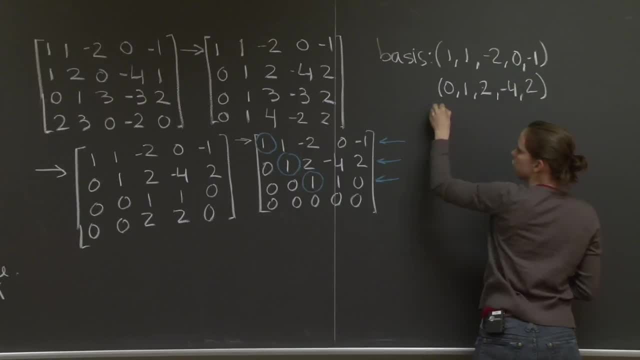 2, 3. 0. 0. 1. 0. 1, 2, 0, 0, 1, 1, 0.. Could you have used the first three rows? Yes, you could. 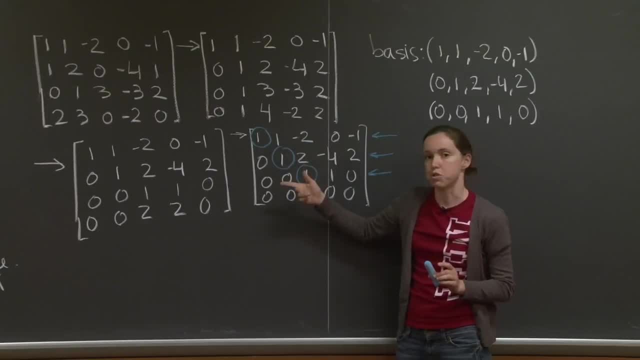 You can't always do that. Sometimes in elimination you have to switch rows because there's a 0 where a pivot should be. When that happens, you have to use these three or you have to keep track of which row you switched. 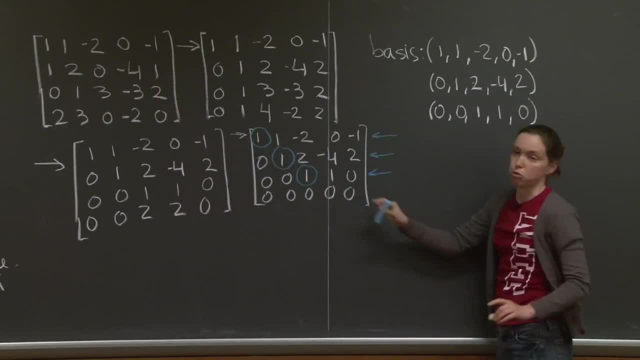 to go back and use the initial ones, But it's really safe to use these ones And also they're simpler than the ones that you started with, so why not? The other question that we had was: what is the dimension of the vector space? 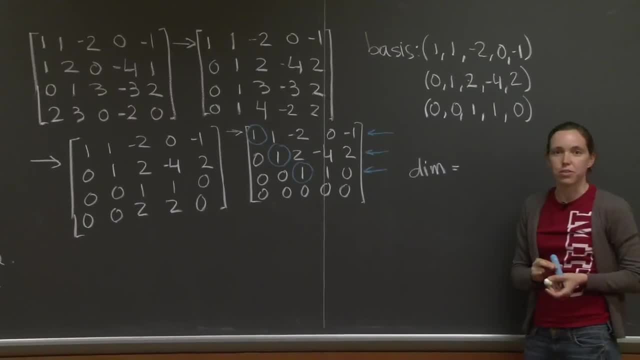 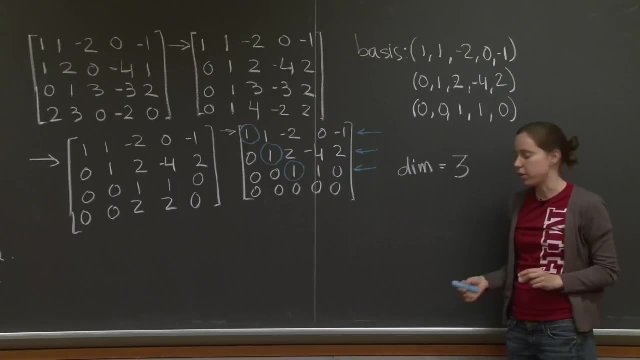 Well, this is the easy part. The dimension of the vector space is 1,, 2,, 3.. And that solves the problem. But there's one more thing that I want to tell you. I told you that there's a couple of ways. 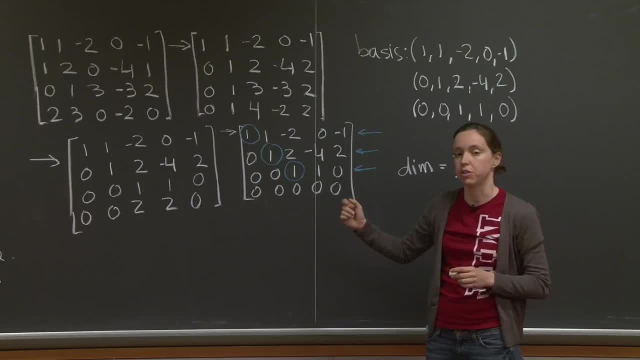 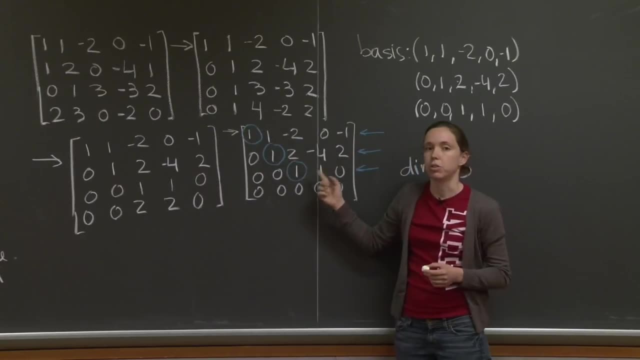 to find out which of those four vectors are linearly independent, And the one that I used was I put them into rows and performed elimination and picked out the rows that have pivots on them. Another way to do it is to write the initial vectors. 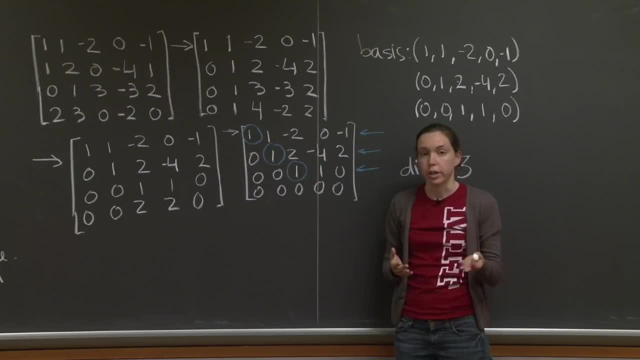 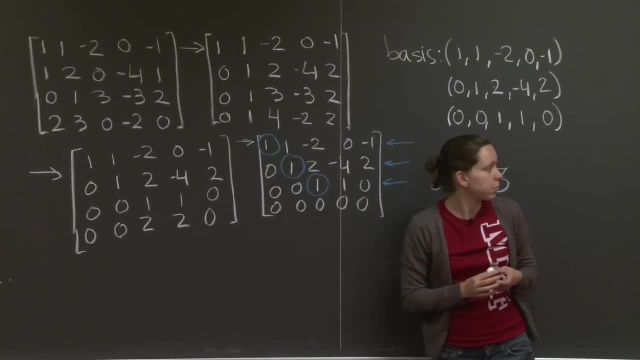 as columns of the matrix and then perform elimination. That also works And, as you know, because you're only working with the transpose of this matrix, you'll get the same number of pivots. Let's go over here, where I have the same, well, the transpose. 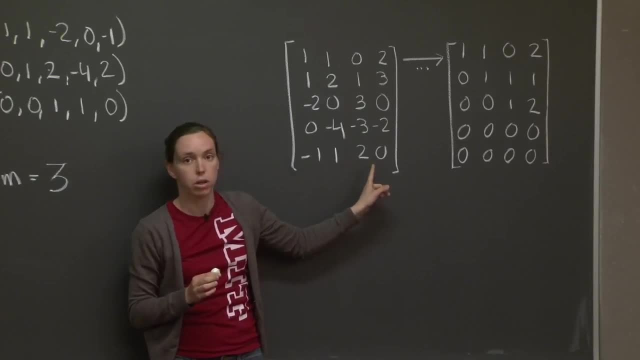 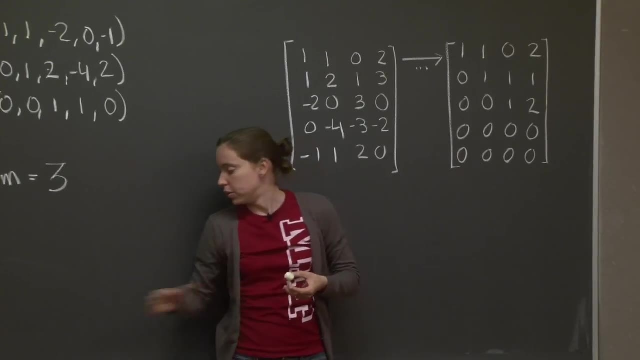 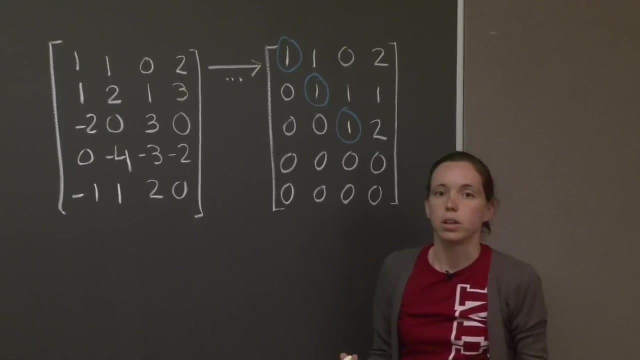 of that, I have the same vectors but now written as columns, My four initial vectors written as columns, And here I have performed elimination And this is the final result. Let me circle the pivots again. Here they are. 3, which is going to give me. 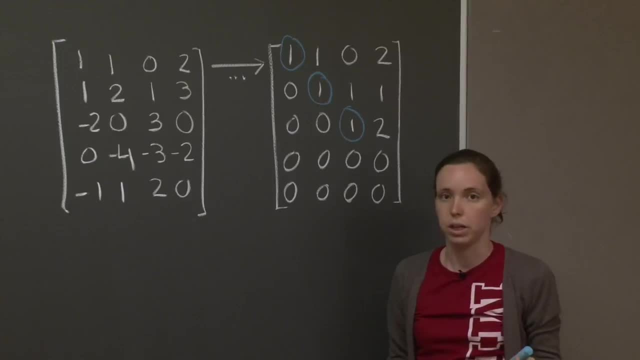 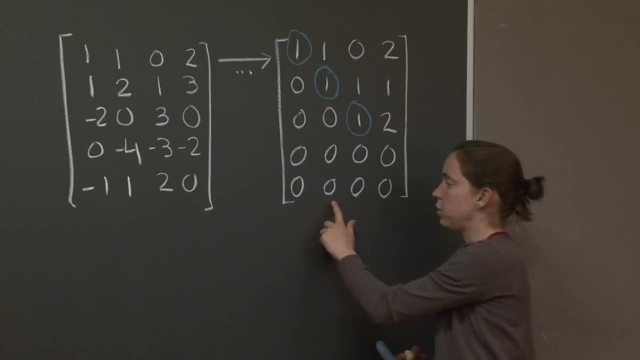 three linearly independent vectors and hence three elements of the basis and hence dimension 3 for the vector space. But I can no longer use these three columns as elements of the basis because when I did elimination I changed the column space. 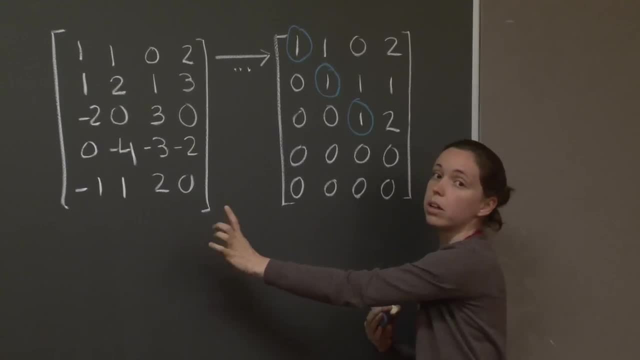 So the column space of this vector, of this matrix is not the same as the column space of the eliminated version. So I cannot use these. In fact, if you look at them, you can probably understand that they're not going to span the same space as these. 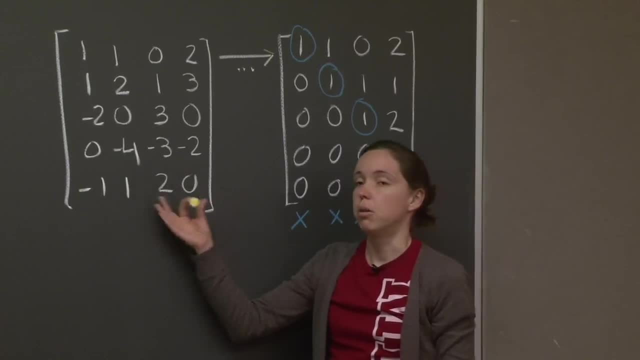 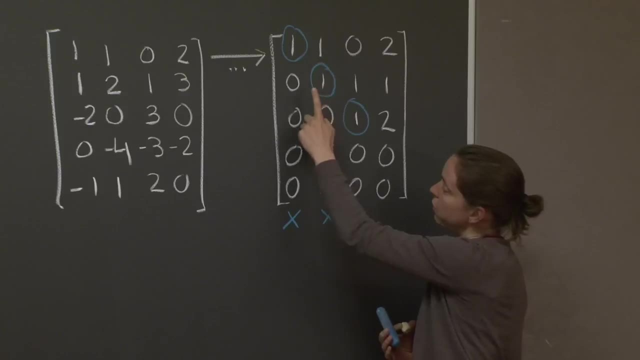 because all that I have down here are zeros, And I get a lot more than just zeros in the last two entries of the vectors. So what I need to do is the pivots are in the first, second and third columns.